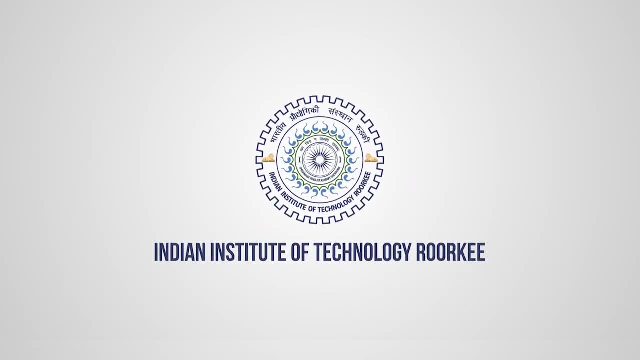 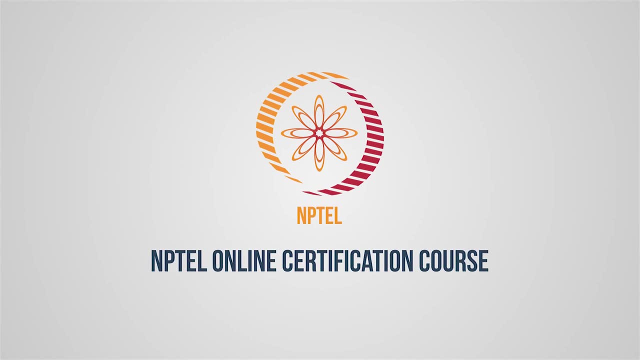 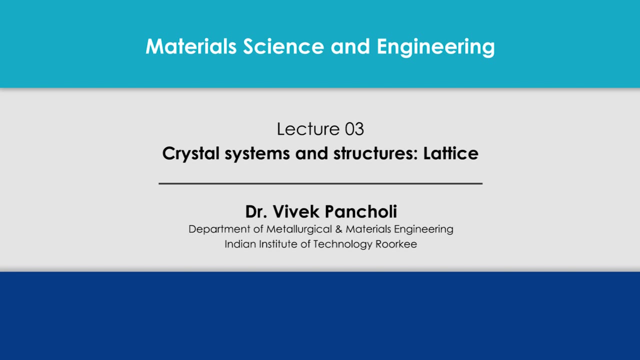 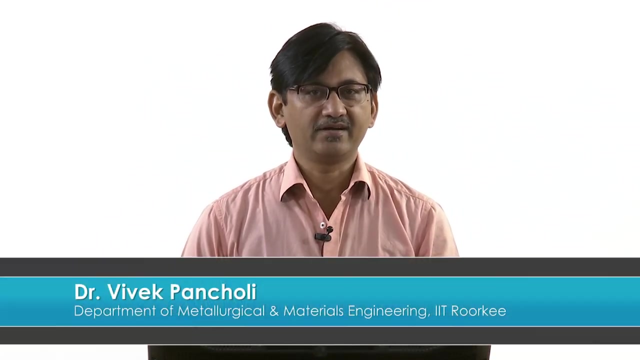 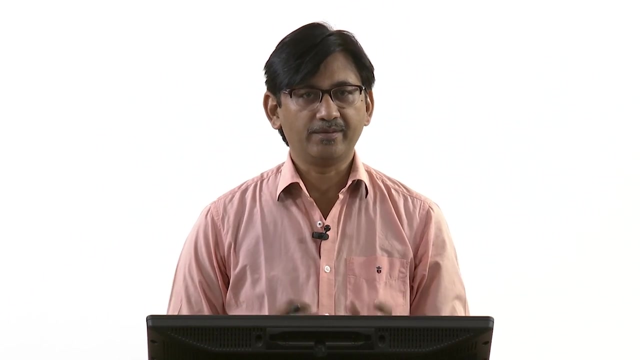 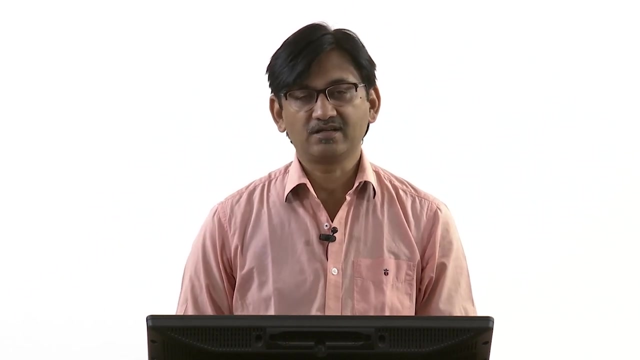 Hello friends, one of the most important to understand the material behaviour is crystal systems and structure. So if we understand the crystal structures we will be able to understand the material behaviour in a much better way, and actually lot of properties depend upon that. what is the crystal structure of the material? So today's lecture we 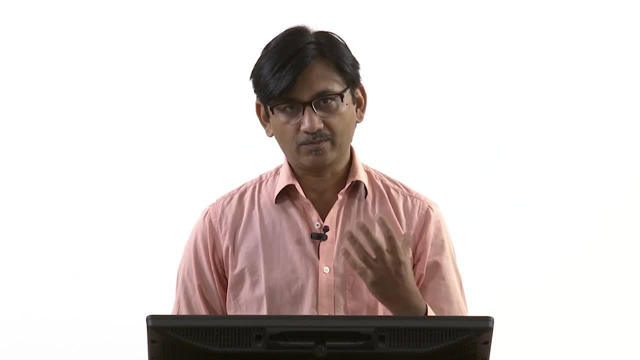 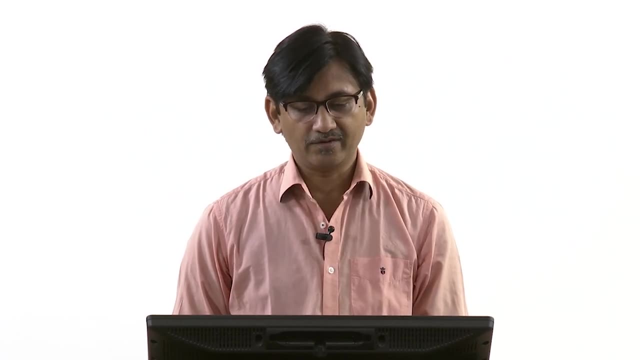 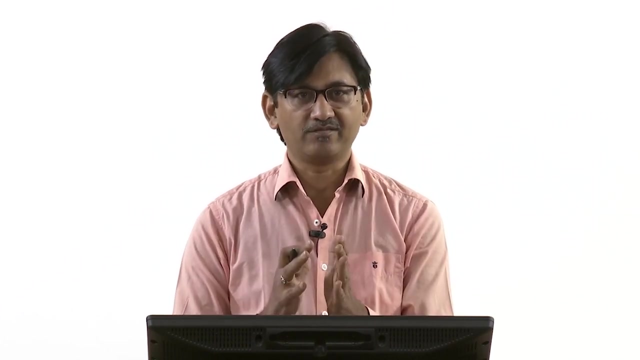 will consider, we will talk about- first we will talk about lattice and then we will come to the crystal systems and crystal structures. So when we want to understand the crystal systems or structures, basically the lattice is the framework which you can use to understand that. what do we mean by crystal system and structures? 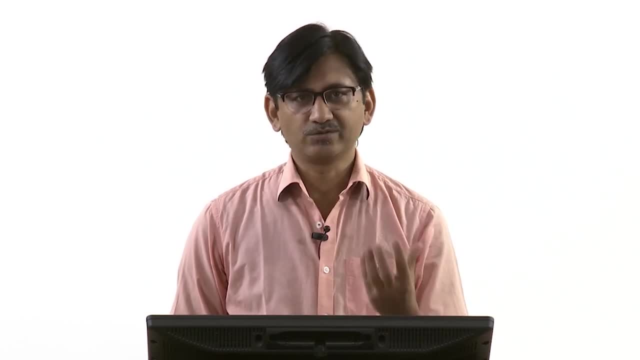 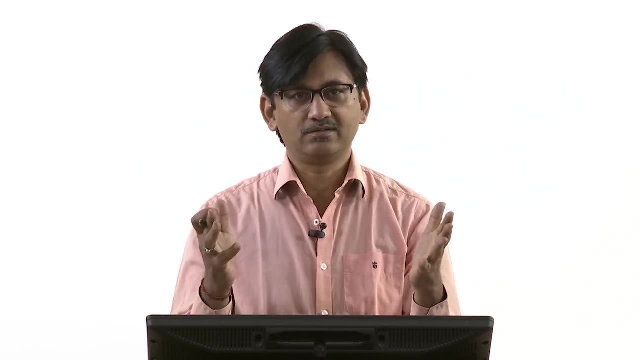 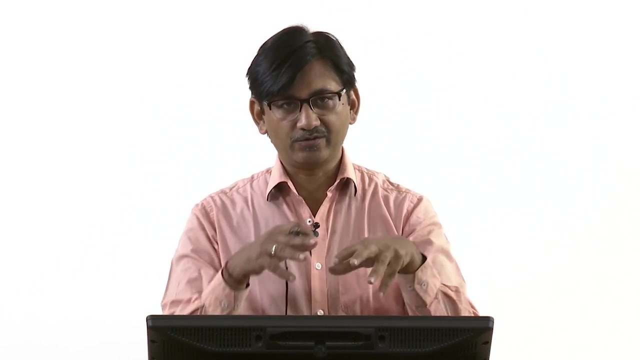 Lattice in loose sense. you must have used a lot of time that whenever you want to, you see a regular pattern. you say that this is a lattice. For example, nowadays you must have seen on the pavements you put those tiles, some very nice shaped tiles, and they 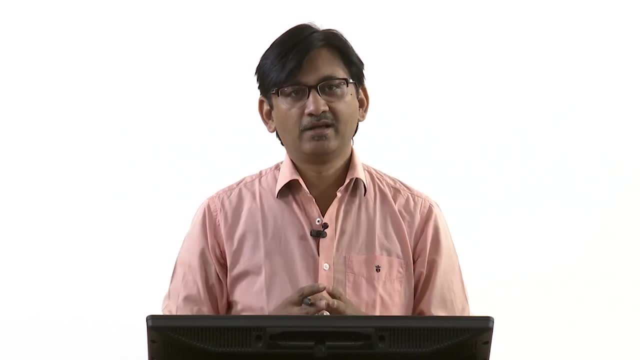 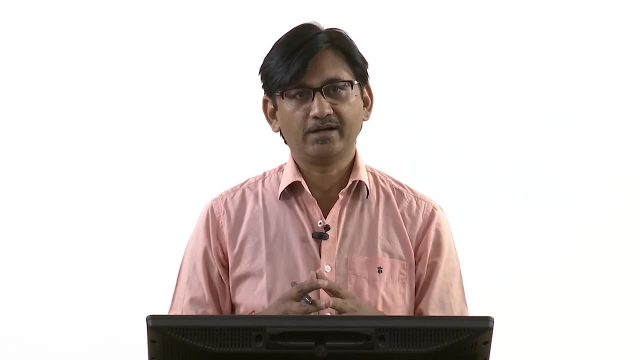 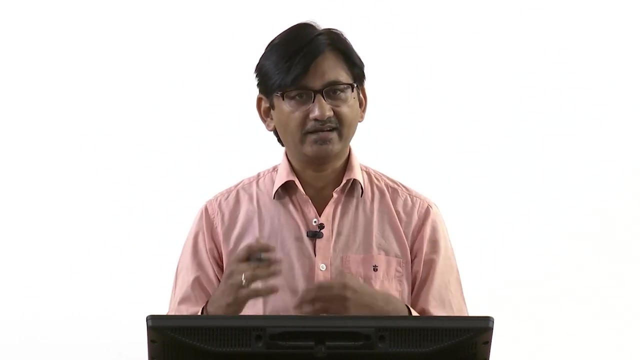 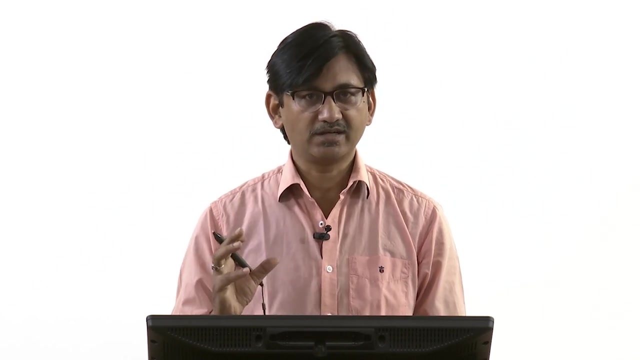 are put next to each other. You must have seen the, or you must have seen the honey bees. they the structure they make, which is a very nice hexagonal lattice. So the lattice is there in the nature and you must have seen it. So the basis for crystal systems and the structure is starts from the lattice. Okay, 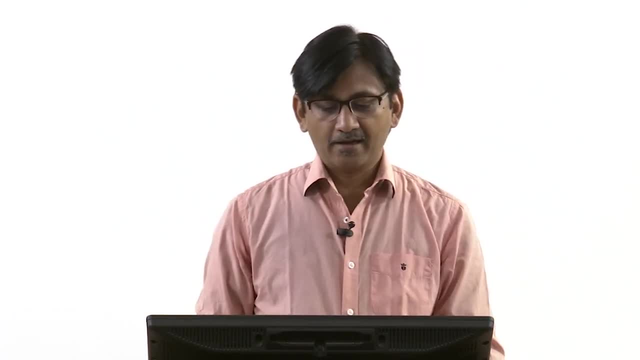 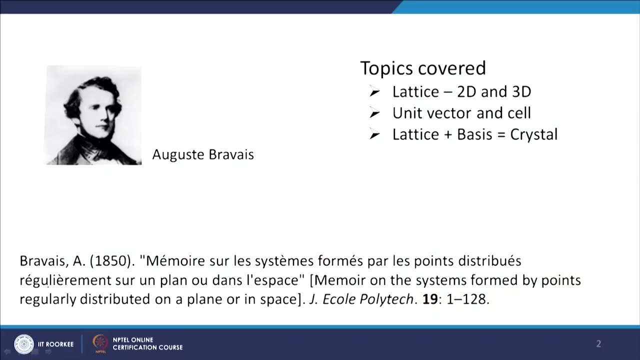 so first let's understand the lattice. this idea was actually proposed by Bravais. that is why they are called Bravais lattices. So in this particular lecture we will cover the lattice in 2D and 3 dimensions and unit vector and cells, And this также we are going to. 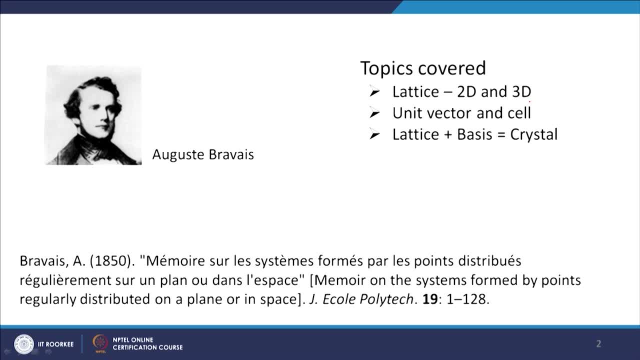 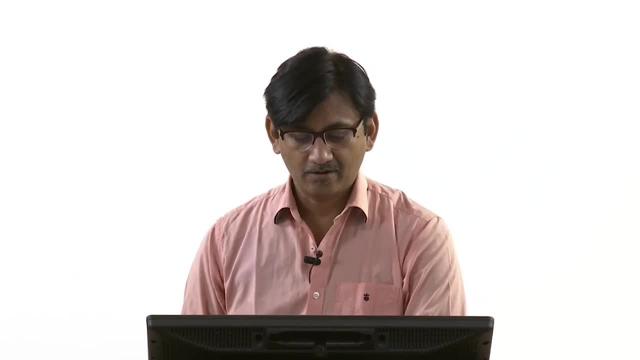 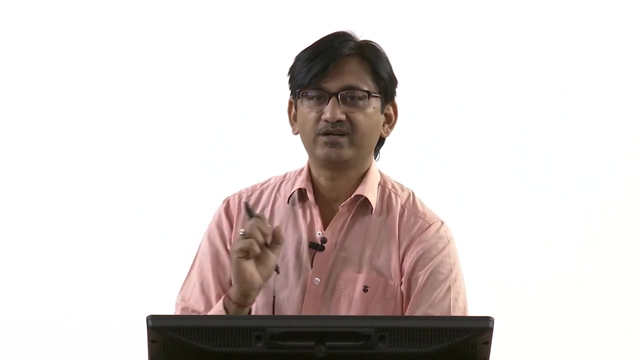 And then we will talk about lattice and plus bases to make crystals. and then what are the different crystal systems and crystal structures? So the Bravais proposed that the idea of lattice and using that idea of lattice, he proposed that there are can be only 7 crystal systems and 14 crystal structures. 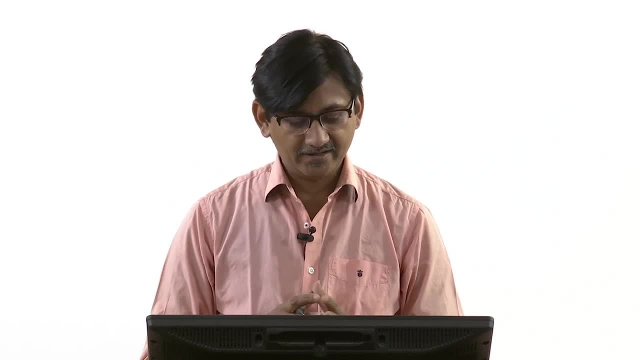 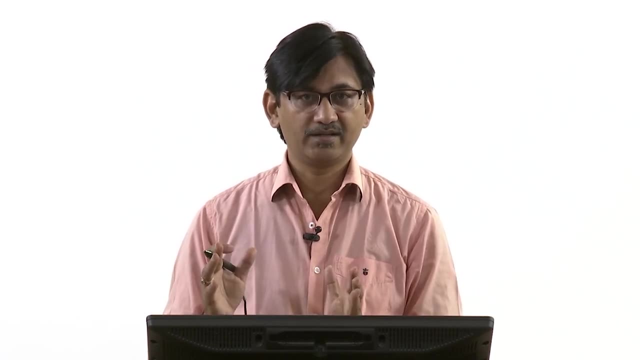 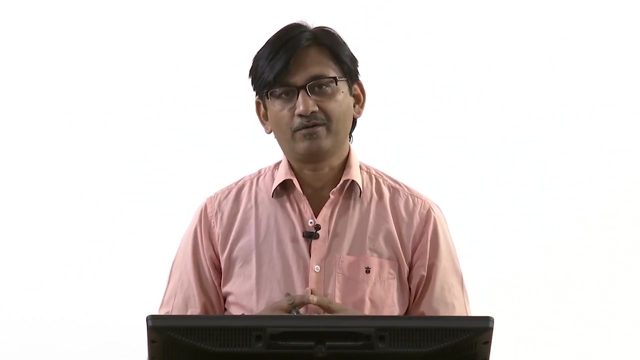 So you can understand and he this work he did in 1850 and you can understand that in at that time he could predict what will be the crystal system and structure in all the natural or main made materials which are possible and they are still. there is no change in that. 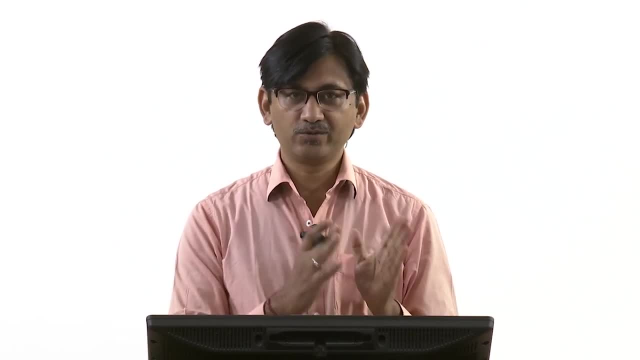 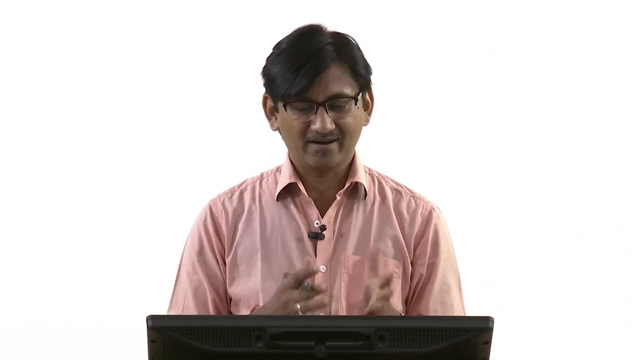 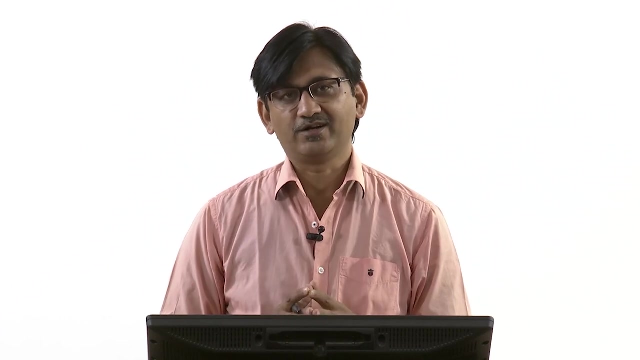 it is still holding and he could do that only by doing geometry. So he must have spent a lot of time And lot of thinking and, of course, he did not have any distractions of TV and your, your smart phones and all that which we nowadays have- all these distractions. 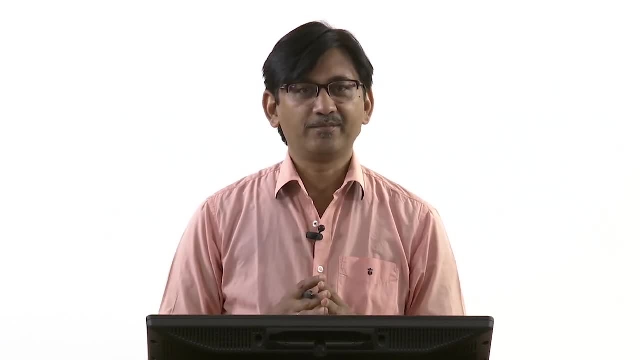 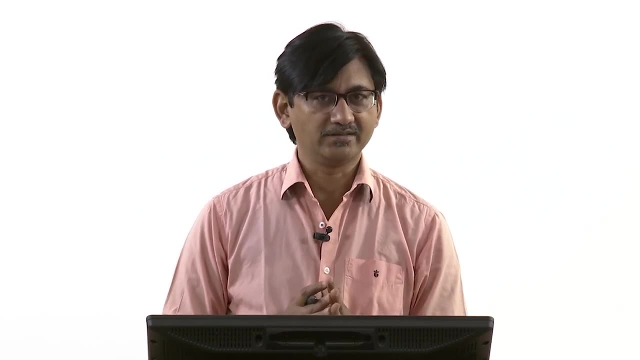 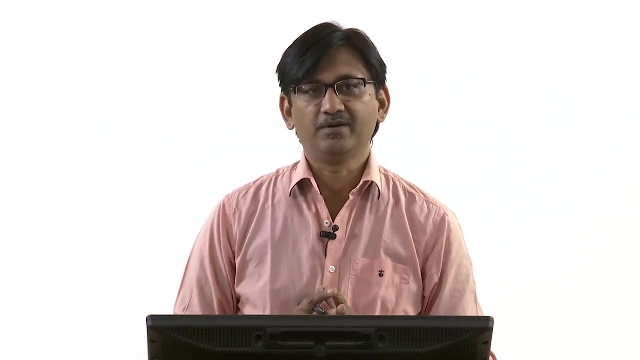 So he did not have that, obviously, and because of that I think he could have devoted lot of time and energy in this concept and using geometry. only he proposed that only these many crystal systems and structures Are possible, and with all the fancy tools which we have nowadays, it is still holding. 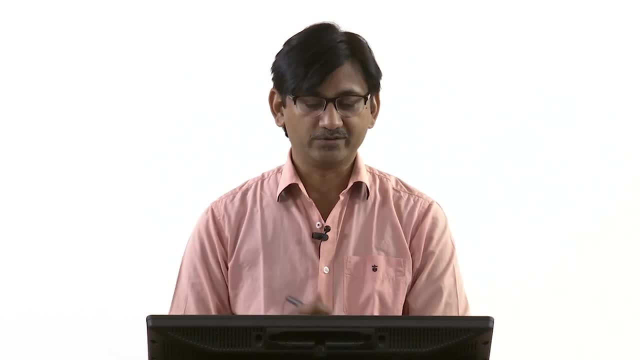 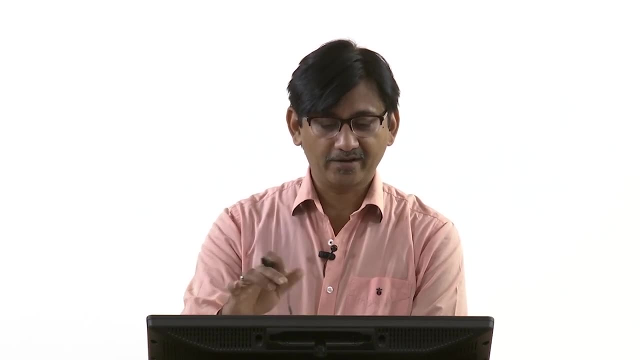 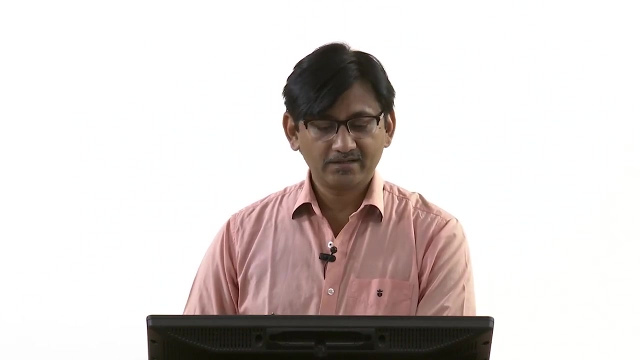 with, we do not have any other than what he proposed in 1850. So the and ideas were very nice and elegant. so, starting from 2D lattice, that. what do we mean by lattice? the important properties of a lattice is that a lattice has exactly same. 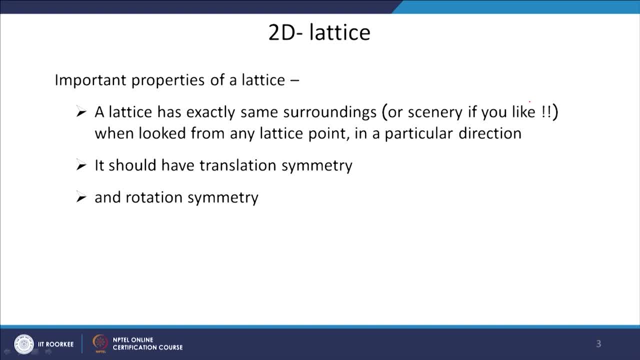 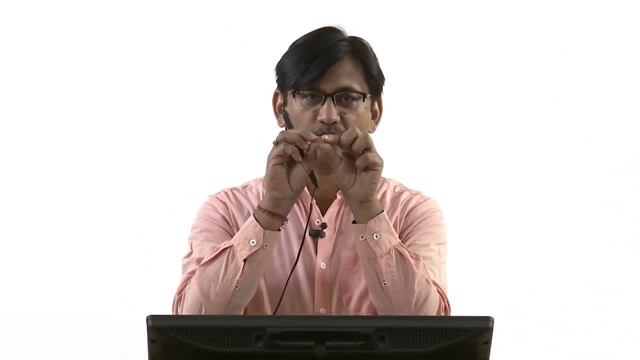 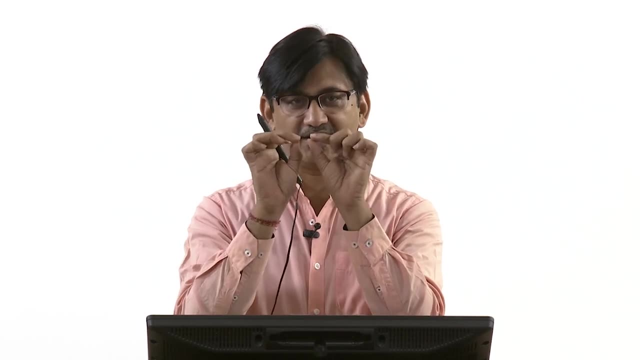 surroundings. This is very important. If you like, you can call it as a same, say: scenery is there. So if you take any lattice point and if you see around that lattice point, other lattice points, if you see, the surrounding has to be same. if I take this lattice point and suppose 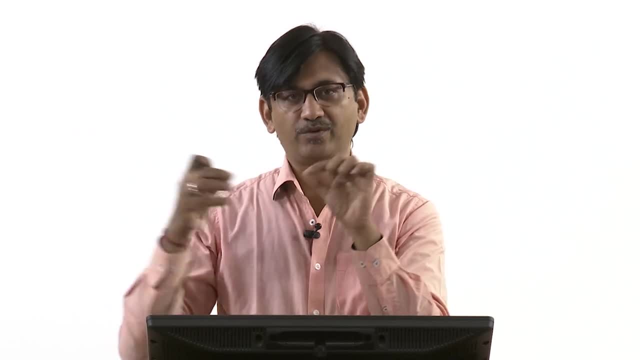 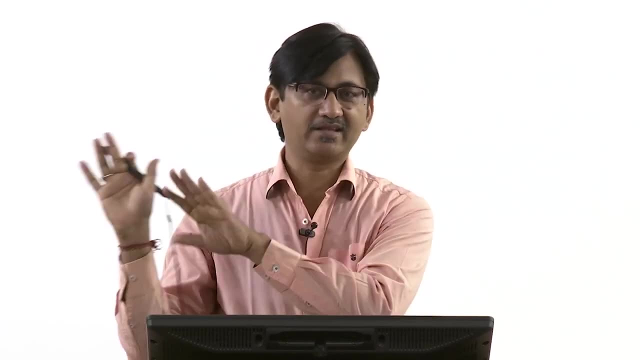 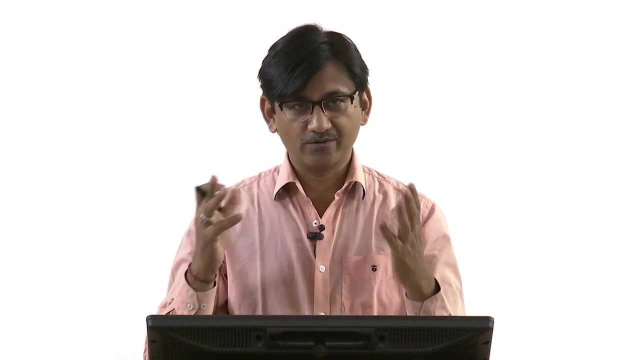 I take may be another lattice point after 10 lattice points, and if I also take surrounding around that lattice point, between this and the new one there should not be any change. It should be same. the scenery has to be same, so the surrounding has to be exactly same. 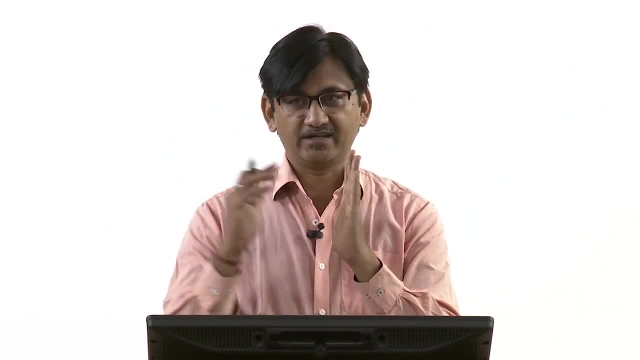 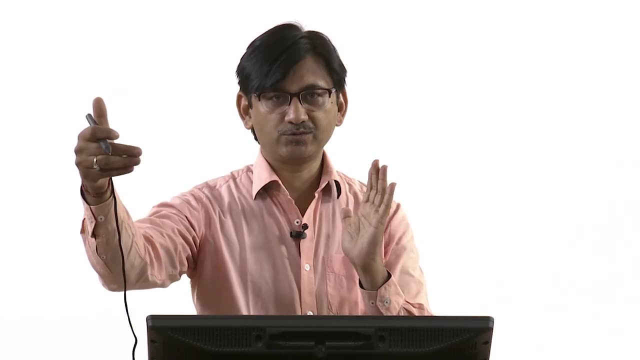 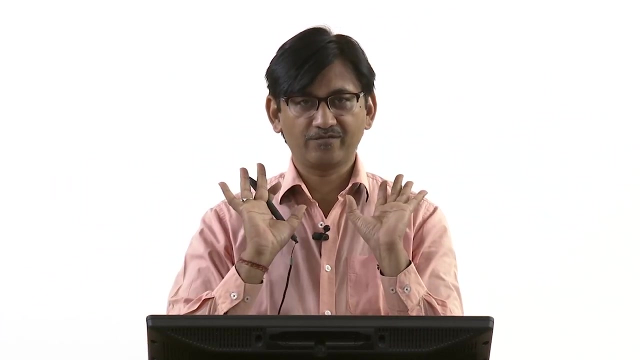 of course you have to look only from one direction. if you want, we are looking from another direction, the surrounding will change, but from that direction, if you see any lattice point, you choose any lattice point, the surrounding around that lattice point will be exactly same. So from looking from one direction, if I choose any lattice point and it can, there can be infinite. 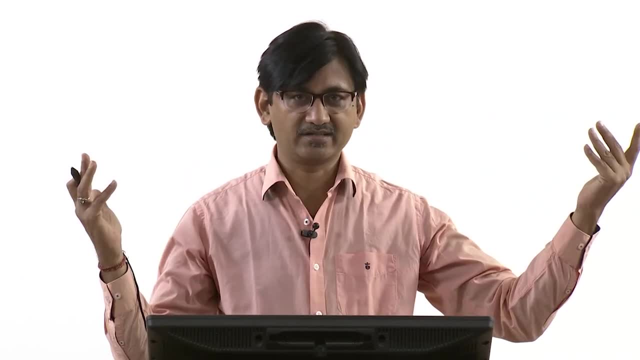 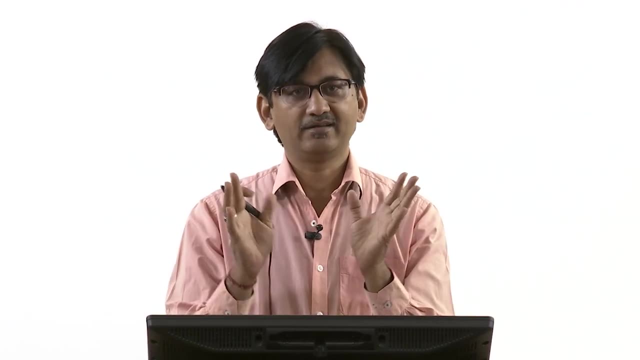 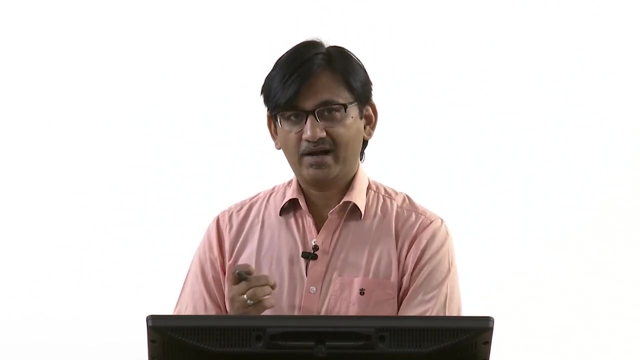 lattice point, So it is a imaginary concept. you can extend it to the length of the universe if you want. you choose any lattice point and around that the surrounding has to be same. So this is the first property it should have. how you can make a lattice is a very simple. 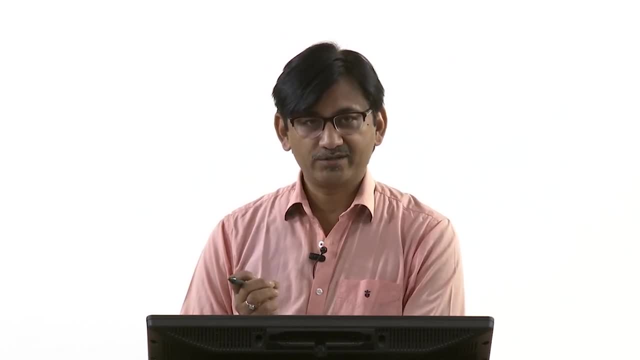 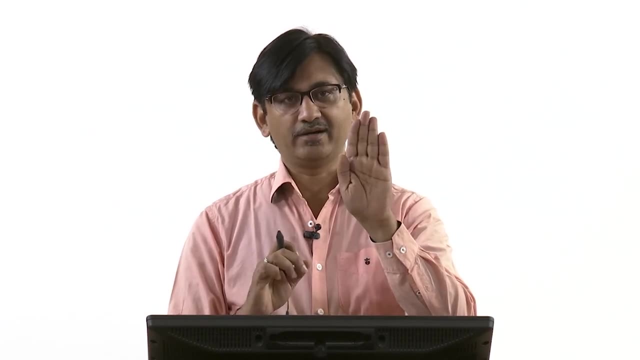 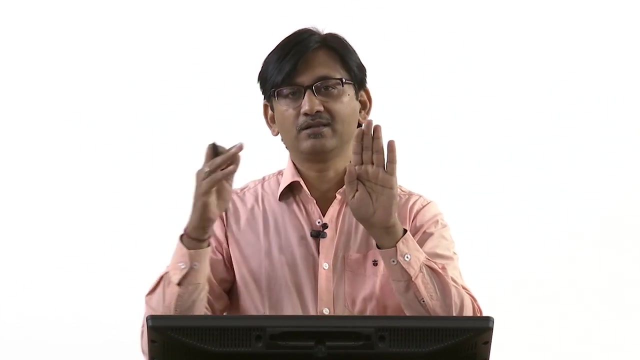 thing, the most important property it should have, is what we call as translation symmetry. So basically, if you have, you start with one lattice point, So you give you two translation vectors in two dimension, then you will be able to get all the lattice points, and up to infinity. 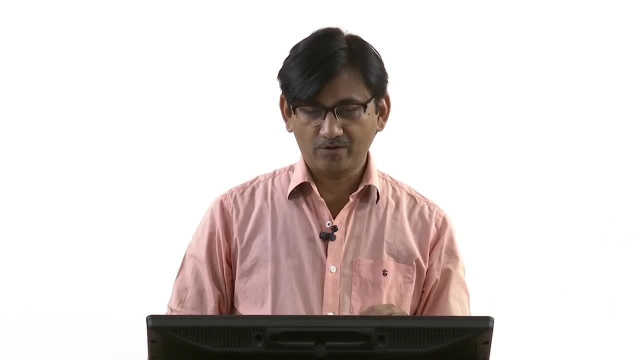 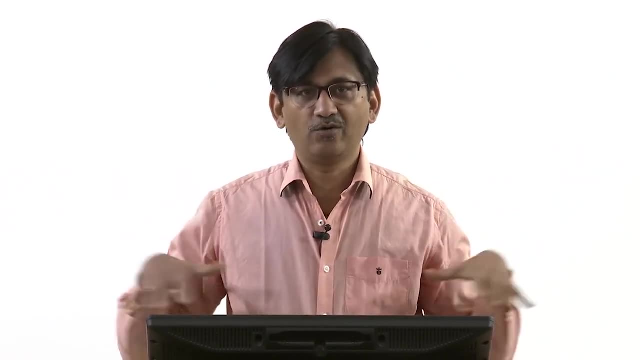 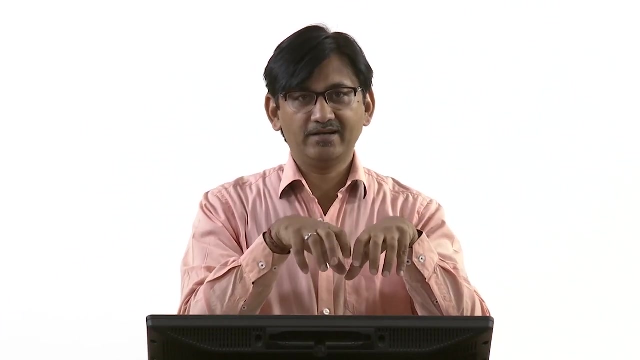 Again, you can take example of the pavement. so if I want to fill the pavement, there is a pavement or any porch is, let us say, and I have to fill the whole area. So what I will do, I will put first tile, then I will put the next tile. so by one translation. 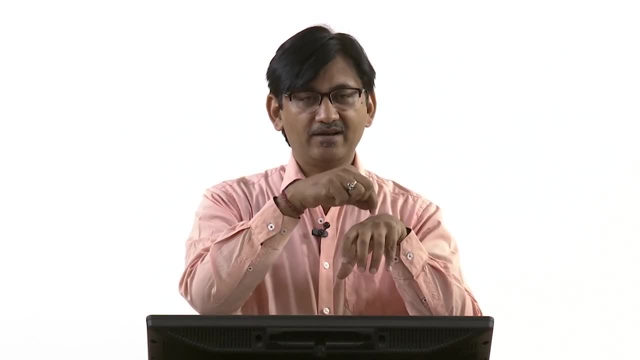 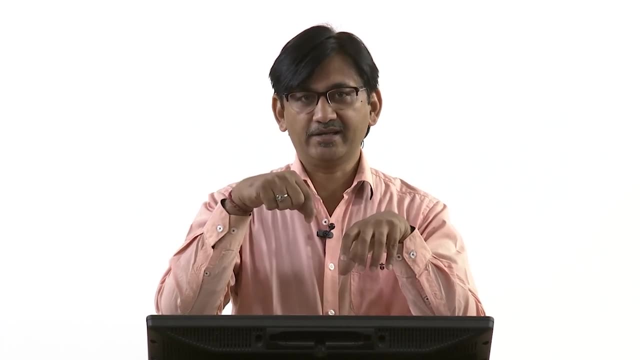 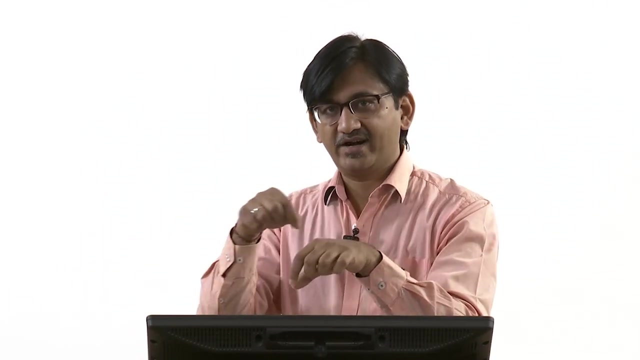 I have put the next tile. so from the centre of the tile, if you see, from this centre to the next tile centre, there is a. you can say it is a vector is there? then I put another tile. So like that, if I keep putting or I can keep translating the vector, then you will get the 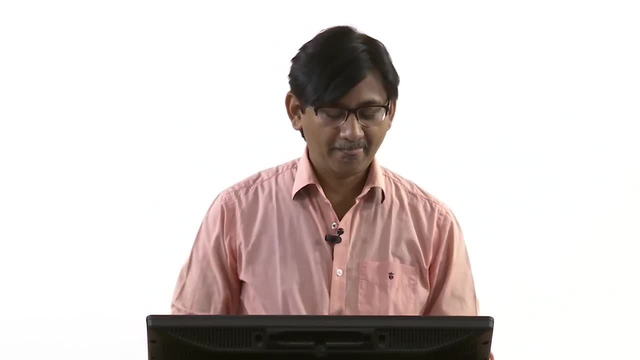 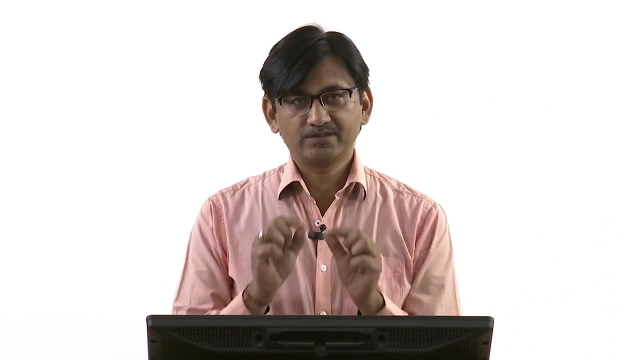 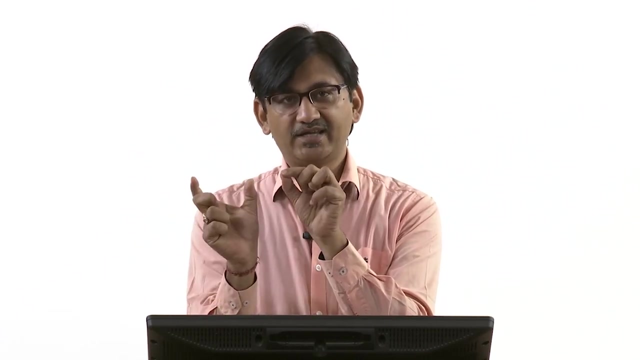 whole area covered and you have a lattice. So in the lattice also the most important property is it should have a translation. That means by translation of one unit vector I should get the next lattice point, another translation of that same unit vector I should get the next lattice point, and so on and that. 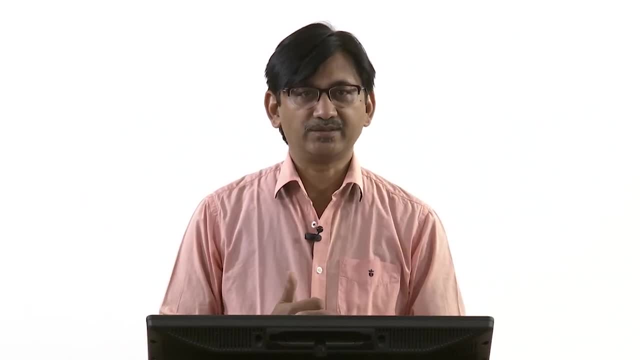 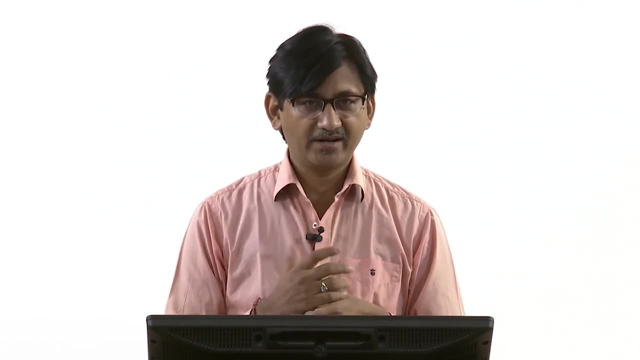 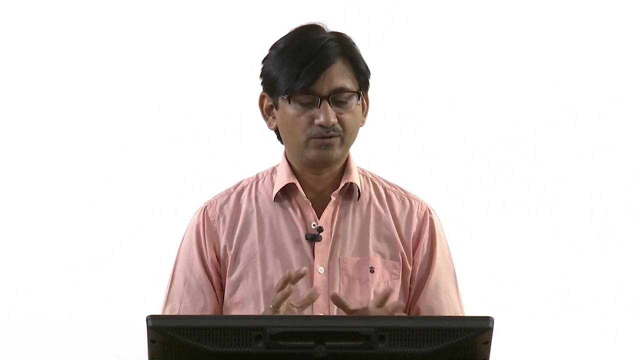 is why the surrounding is same, because it has a translation symmetry everywhere the translation has to be same. okay, the translation vector has to be same. Another very important property it should have is called rotation symmetry. we will not cover rotation symmetry too much, okay, but we will use translation symmetry to understand the 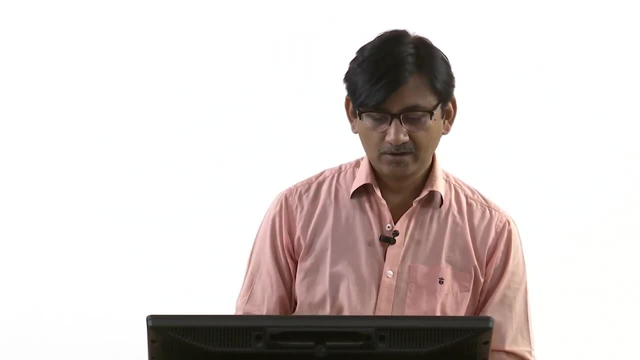 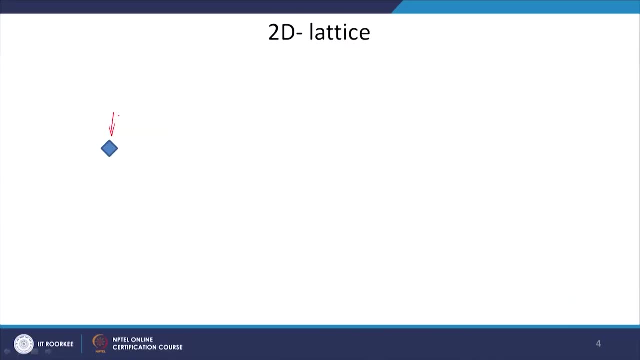 lattice and to construct a lattice. okay, So like, let us start with a with a lattice point like that. okay, so this is a lattice point and we want to create a two dimensional lattice. okay, and suppose I have defined unit vector A in this direction and suppose I so when I translate it by A in that direction. 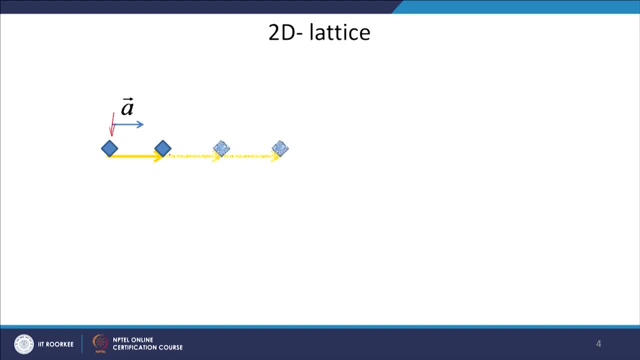 I should get the next lattice point- okay. similarly, if I keep translating, I should get the next lattice point by the same vector A- okay. similarly, I can have another vector B- okay, in another direction. and if I keep translating by vector B in another direction, I should get the next. 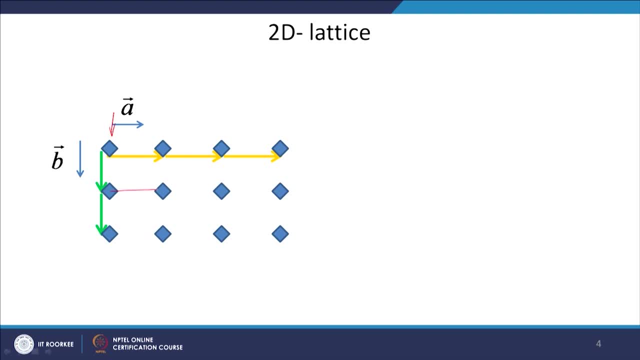 lattice point. So if I do a vector translation of this A, it should have been little bit larger here, okay, so by doing a translation of A, I should get the next lattice point in this direction, in the direction of A, if I keep translating by a vector B in this direction, in the direction. 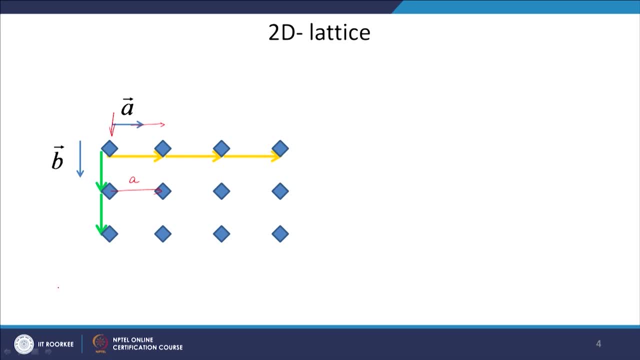 of B, I should get the next lattice point And if I keep doing that I will fill the whole area here. okay, and I should get the lattice point and if you see the surrounding, as I was telling you suppose you choose this lattice point if I check the surrounding. okay, so you have one lattice point here, another here and 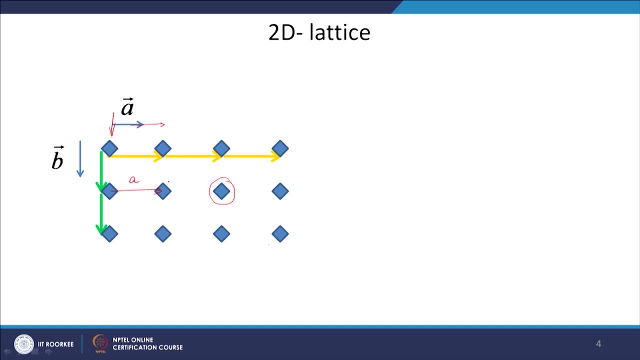 the distances they look very same. then what? I suppose I choose this lattice point again. the surrounding is same. so for each lattice point the surrounding is same, and that is because you have this translation symmetry. okay, So this translations vector can be easily represented by a mathematical equation like: